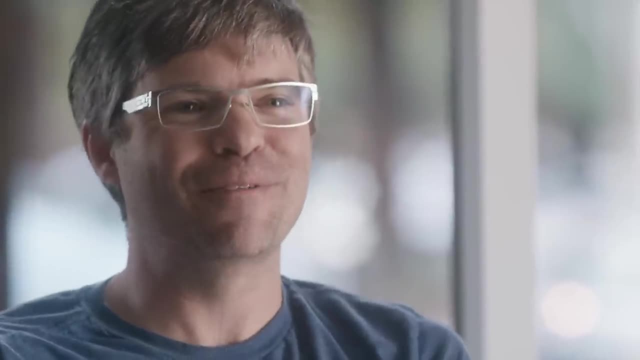 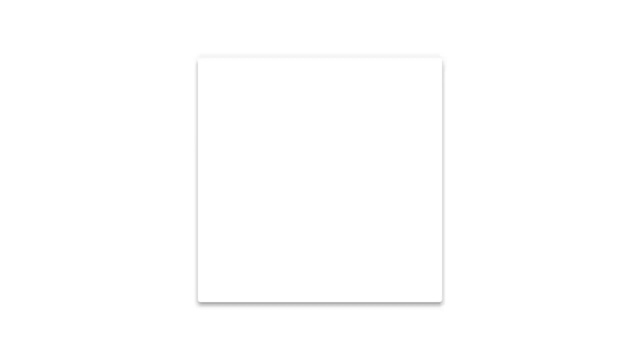 what is this made of? What is the material that our software is made of? John came up with the idea of what he described as quantum paper in order to create these rich tactile user interfaces, And that idea of it being mostly paper-like but smart paper. 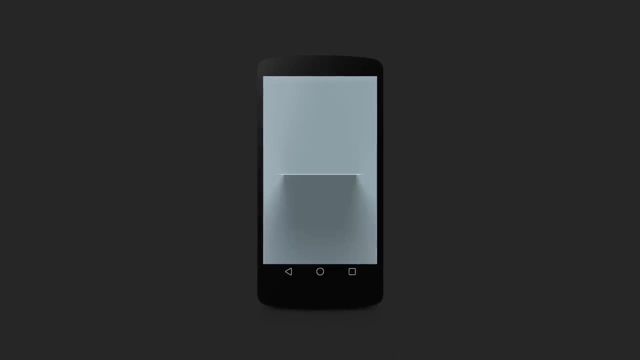 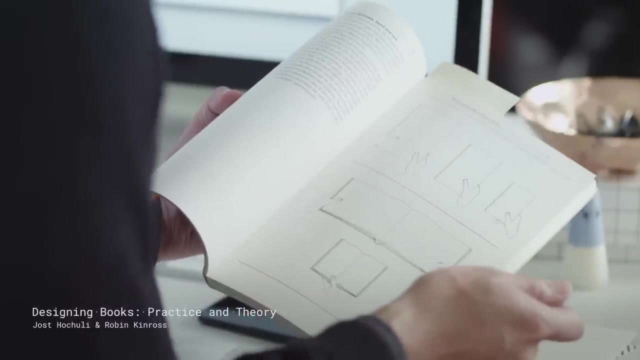 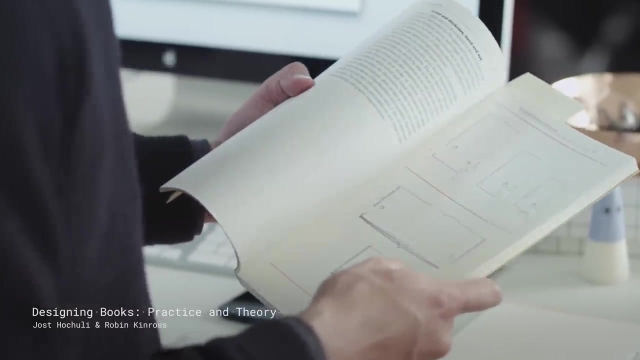 served as a point of view about how your surfaces work and why There's a very, very clear parallel between the systems of book design and the way that you know, humans also hold and use devices. People use materials in life every day and we want them to understand software in the same way. 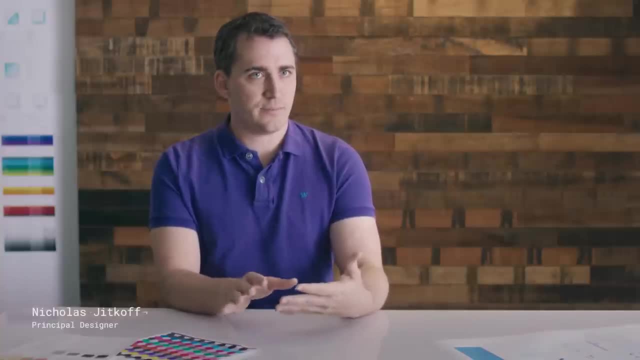 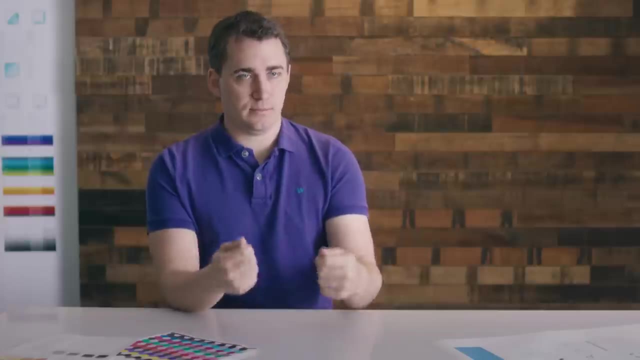 When we're thinking about how a digital surface works, think about all the different shortcomings and advantages it has. One of the main things that we run into is that you have this sort of flat plate of glass, which is great because it's easy to move around. 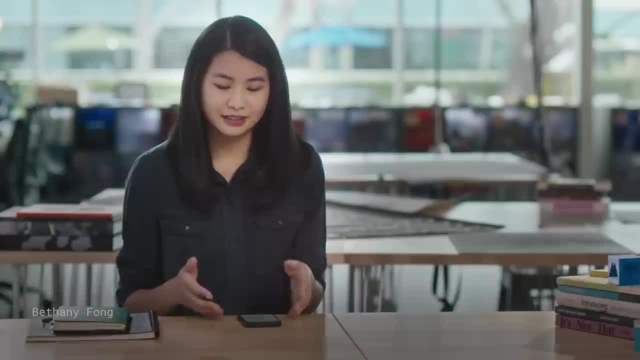 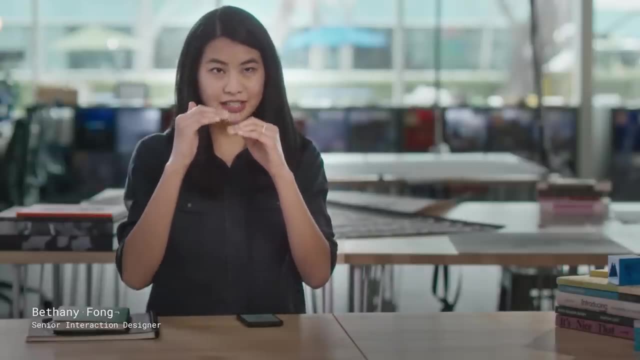 but it also prevents you from actually being able to touch the things that you're working with. Inside this device, there is actually a little bit of space, And so we thought, well, let's try and take advantage. Let's take advantage of that and create a meaningful structure that goes underneath it. 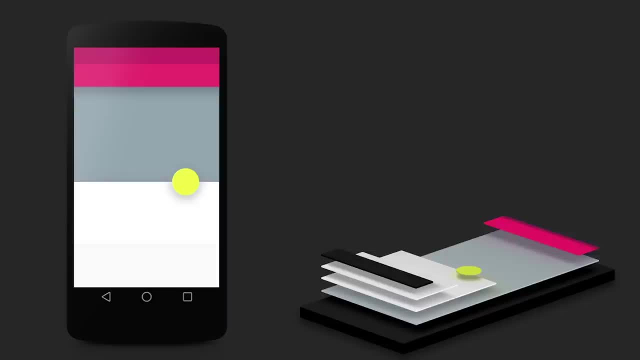 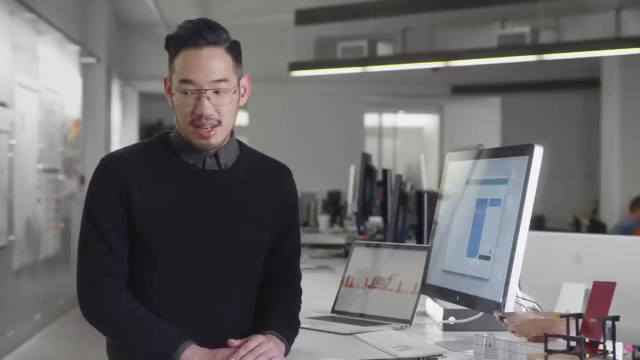 almost like the skeleton filling out this body from the inside out. Material design early on was almost like we were going out and trying experiments. Yeah, it was totally an experiment. Everyone kind of sat next to each other in a room working on all the different aspects and components together. 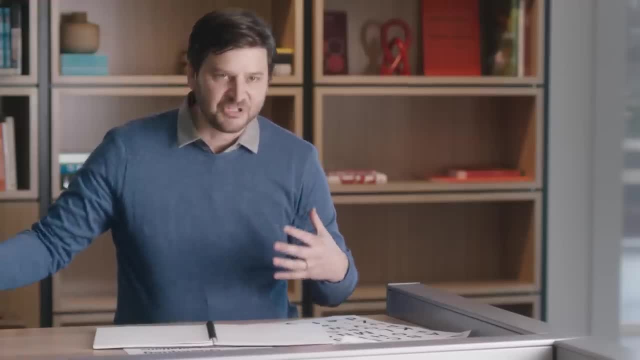 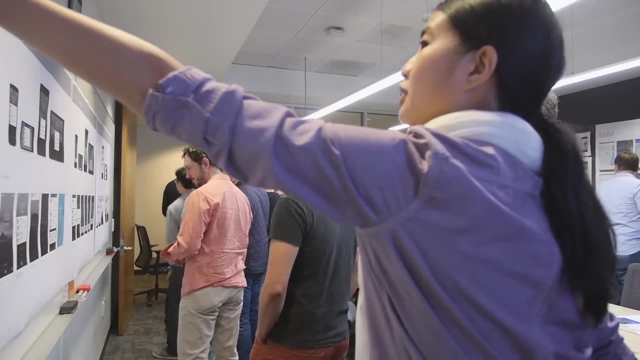 Kind of riffing off of each other. It's one thing to play by yourself. It's another thing to play in a group where you're improvising in real time. I think a lot of us are used to working more practically. This is the first time where we're being pushed and told. 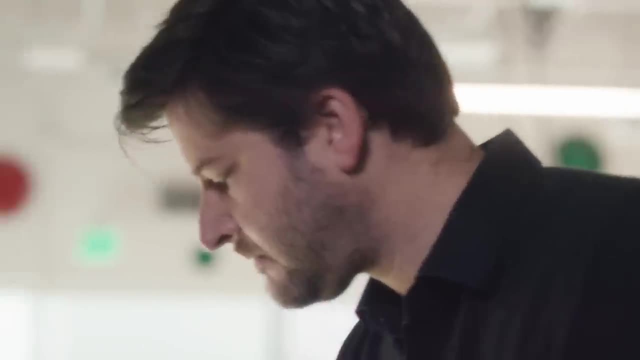 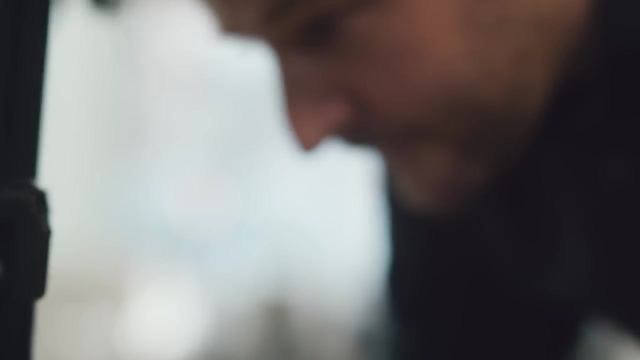 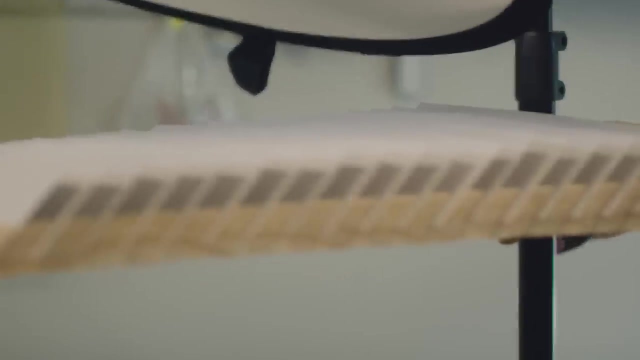 don't worry about that. Let's just see what happens now. Yeah, so this is something that we've done a few times. We've set up these light rigs to understand how the shadows work. The depth cues that come from the shadows really made us think more deeply about. 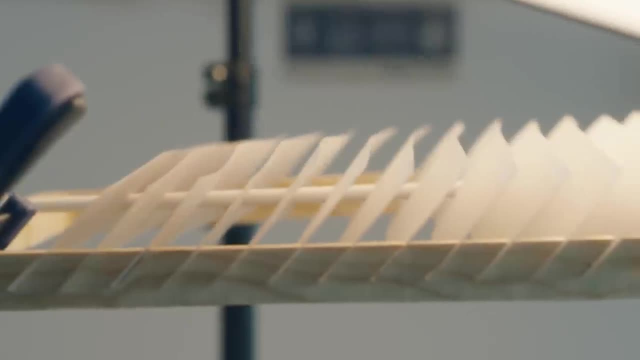 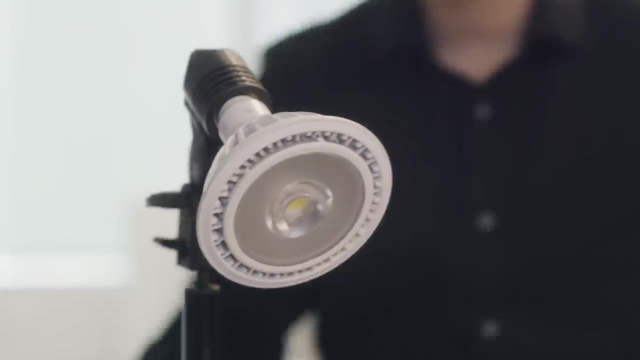 how do we communicate surface? We built a system that enforces that the light comes in at 45 degrees, So we can see the light coming in at 45 degrees. We've got a lot of different degree angles. that helps keep the shadows consistent from. 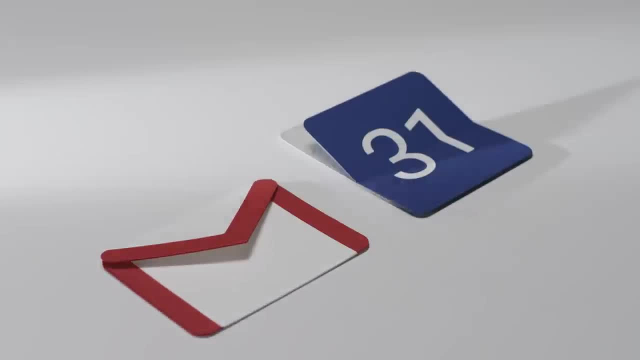 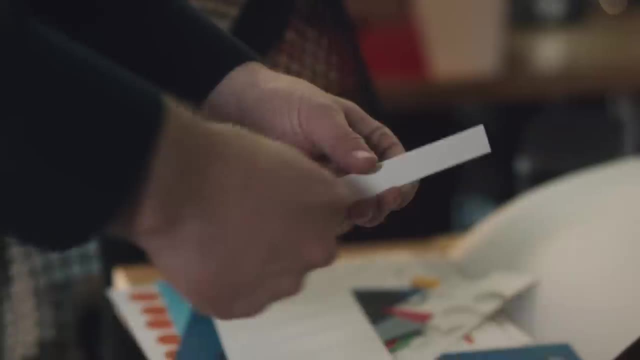 the top to the bottom of the screen. Even as we were designing out the icons, we started to see some really interesting subtleties you wouldn't normally notice, but these are things we pick up on and help us to understand that it's a surface. 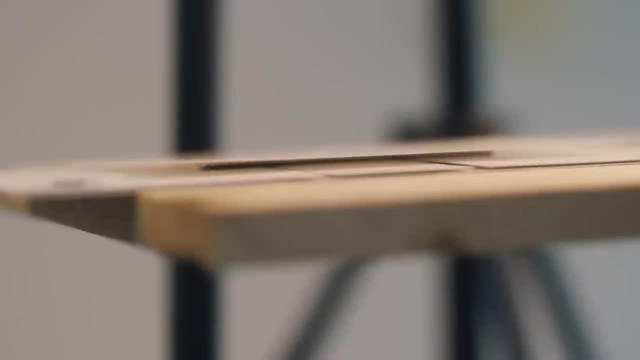 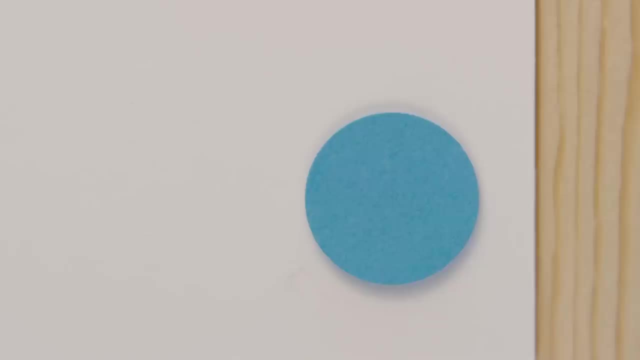 Strips are spacers measured out to scale, to the way that they're modeled digitally, So not just X and Y, but also in Z. When we were creating Action Button, the FAB, the way that we said. there's just one thing. 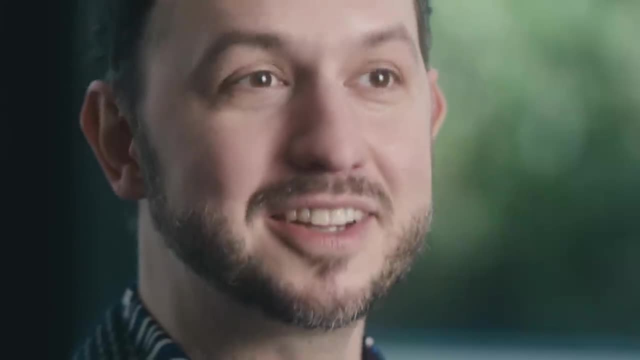 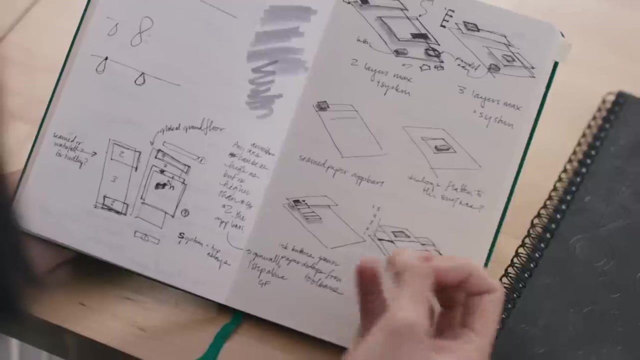 stop with your five buttons. your four buttons make the call. I thought that was great, And it was not an idea that I was comfortable with at first. Button sounds like such a simple concept, though when we kind of took it down to its. 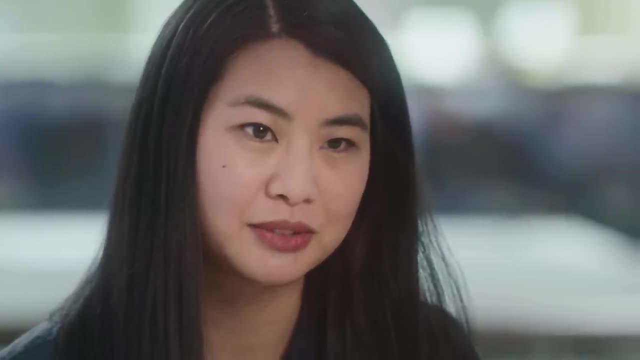 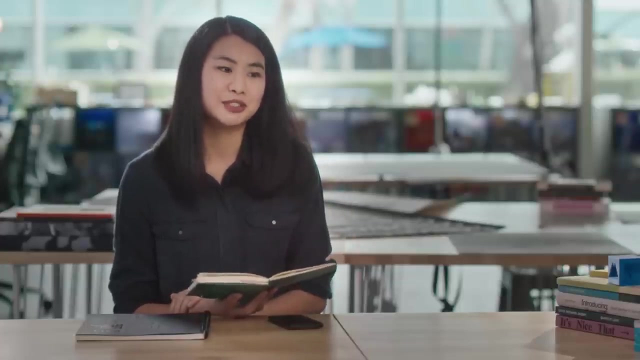 basics of well, it's this area on screen that lets a user perform an action. it's this very concentrated thing that should make the user feel powerful And like they're able to complete something. There were little things like having buttons that depressed felt a little bit odd, because 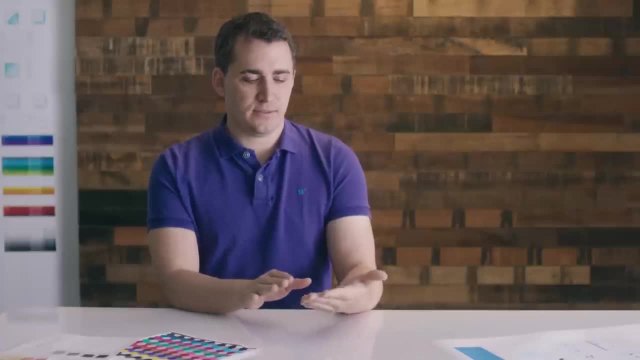 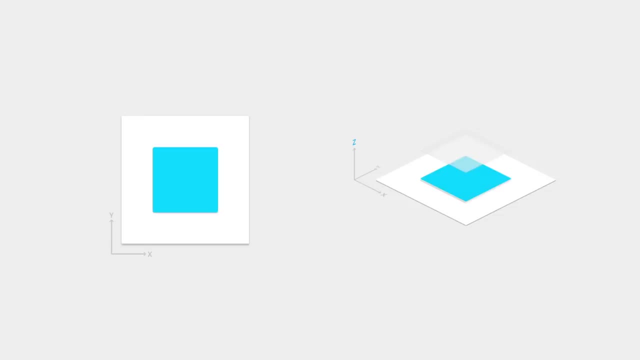 they're not actually depressing. Your finger doesn't feel anything moving down And in fact this like millimeter layer of glass between you and the actual image means that you're not even getting to it in the first place. So instead we reversed it. 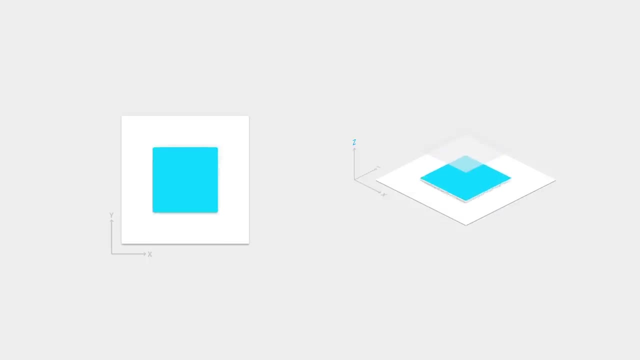 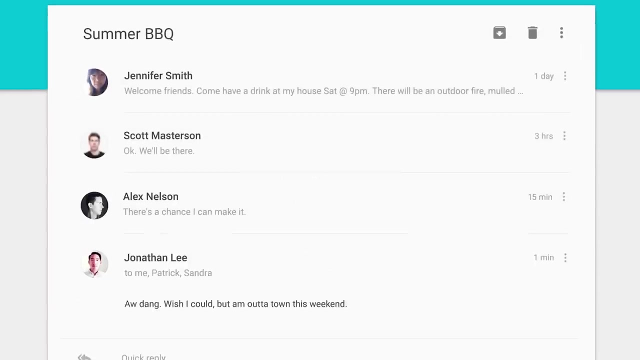 So we had buttons that lifted up when you touched them, So it was more of a magnetic attraction of your finger. There's a logic to it, but also a magic in it. Past the motion, there was the graphic design aspect, the boldness, the typography, the 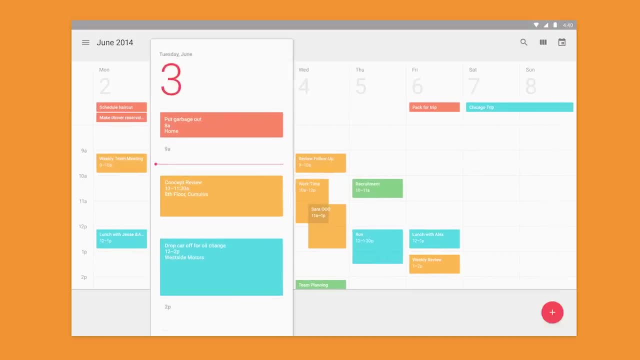 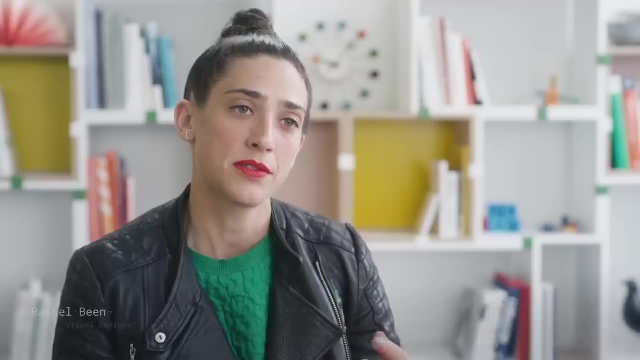 imagery. Those were all in there. We also intended to give the system a bit more robustness. You want people to feel comfortable with it, but we wanted to feel very well designed. We created this color spectrum around picking sort of a primary color and then using an. 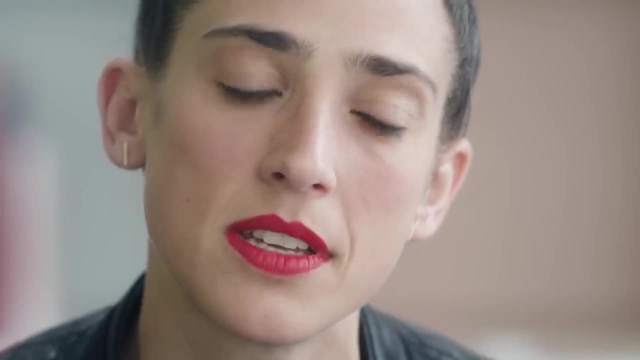 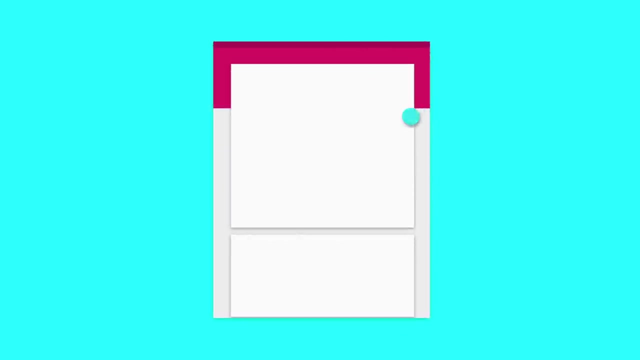 accent color, creating this really simplified and easy to use system while being very definitive. Someone who never took a color theory class could create a combination of colors within their product that felt harmonious. I design fonts, and one of the things that I really like about that- 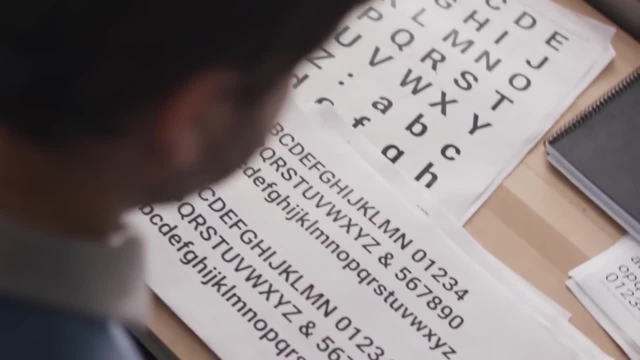 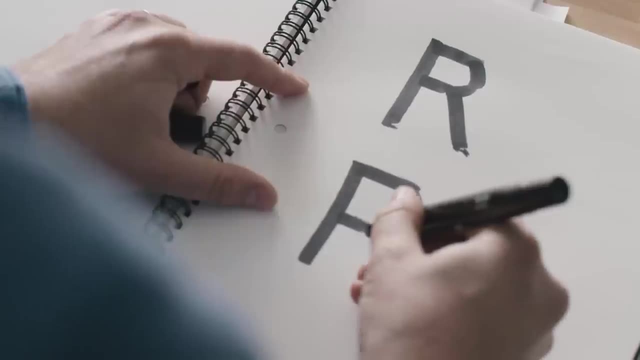 is, the font doesn't come to life until another person uses it, And we really see Roboto as a living typeface that you know as needs change and as we introduce new form factors, as we need it to do more things, we can continue to revise.